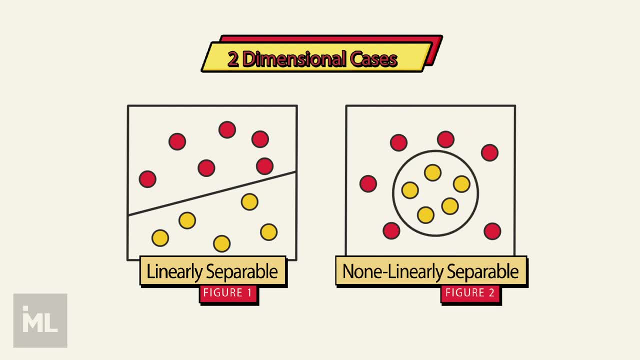 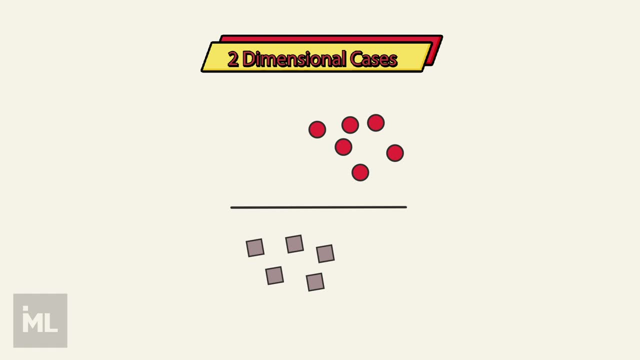 which means that we cannot find a line to separate the data. Therefore, we say the data are linearly separable. Figure 3 shows that the data are linearly separable if we can find a line to separate the original data. Let's have a closer look at Figure 1.. In general, there are lots of possible solutions for drawing. 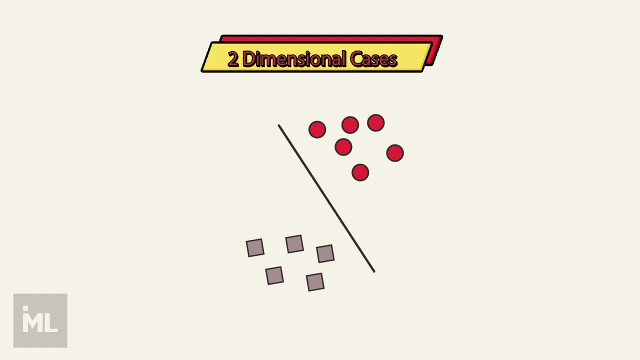 a hyperplane to separate the positive samples from the negative samples. But which one is the best? SVM can help us choose the best hyperplane which maximize the margin, or sometimes we call it a straight around the hyperplane to separate the positive ones from the negative ones. 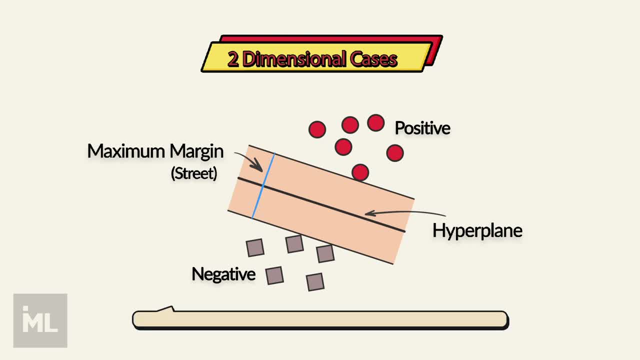 That's the reason why sometimes we also call SVM the maximum margin classifier. Now let's introduce another important concept: support vectors. Support vectors are the data points that lie closest to the hyperplane. They are the data points most difficult to classify. 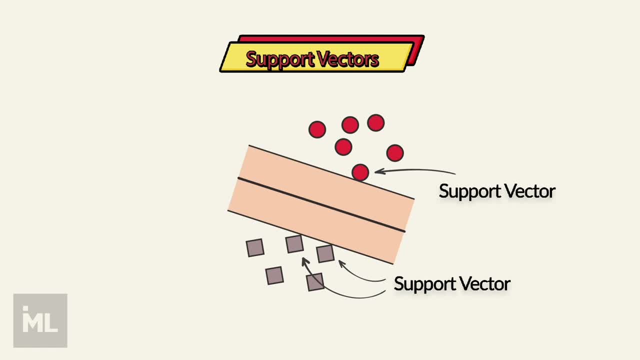 which also decide which hyperplane we should choose. Unlike some other machine learning models, like linear regression, we can also draw a line to separate the positive and negative samples. For SVM, only the difficult points, which is, the support vectors, has an impact on the final. 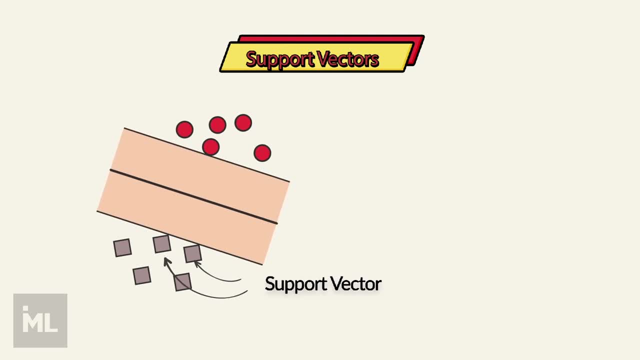 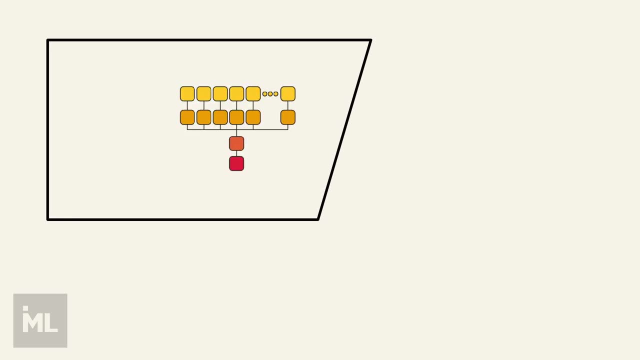 decision boundary. Moving a support vector moves the decision boundary. Moving the other vectors has no impact. Just like any other machine learning model, during the inference time, SVM will predict the output y with input x. The input is just a set of features. 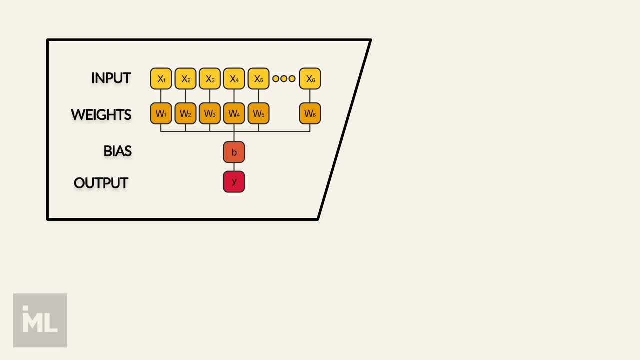 x for each sample. SVM will help us to find a set of weights- w- for each feature. Then, through the linear combination of input features and weights, we can predict the output y. So far it is just like the neural net. However, there is a major difference: SVM will optimize. 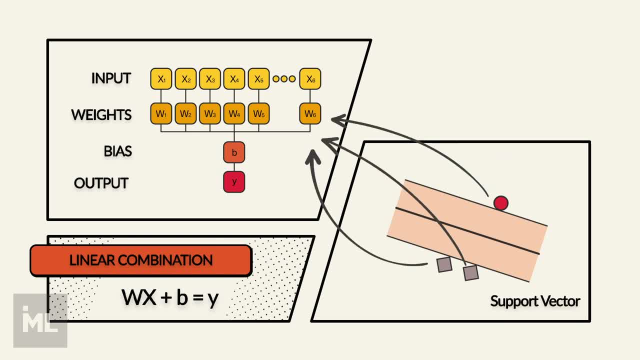 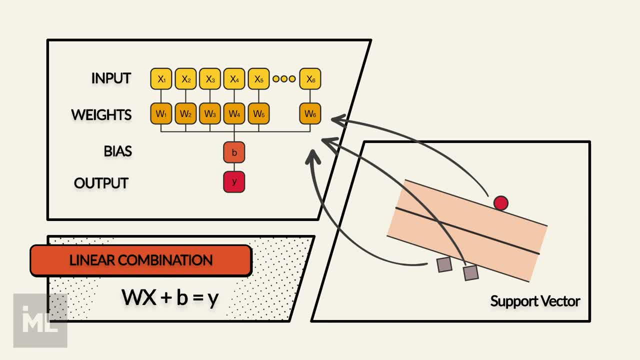 fun part of SVM. Let's start the fun part of SVM. Let's start the fun part of SVM. We are going to go through the underlying mathematical process for SVM to find the hyperplane and maximum the margin. This part only requires that you have some basic background of linear algebra. 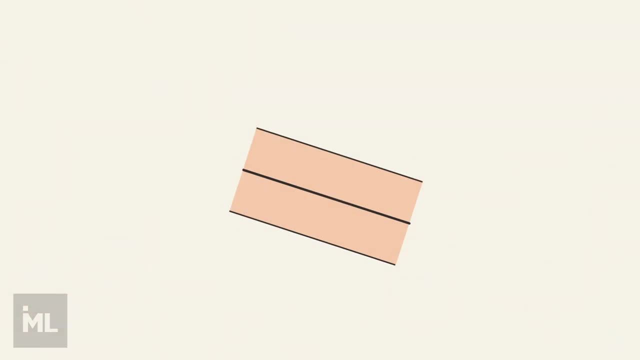 and optimization theory. Still for this 2D example, we have three important lines: The middle line of the straight H0, which is the hyperplane, Two gutters of the straight H1 and H2.. Now let's assume there is a vector w perpendicular to these three lines, For all the points on H0,. 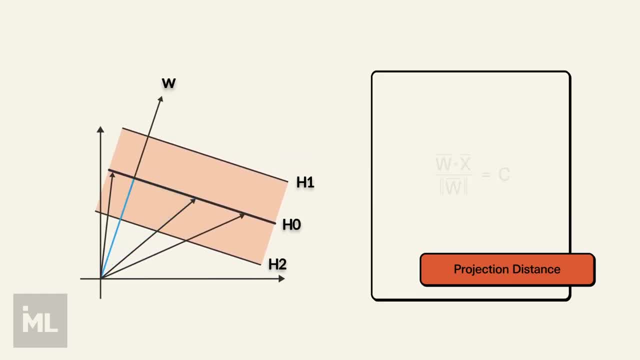 they should have the same projection distance on w direction, which is w dotted x over the magnitude of w is equal to c. Let's multiply the magnitude of w on each side of the equation. We can obtain w dotted x is equal to c times the magnitude of w. Now let's substitute c times the magnitude of w. 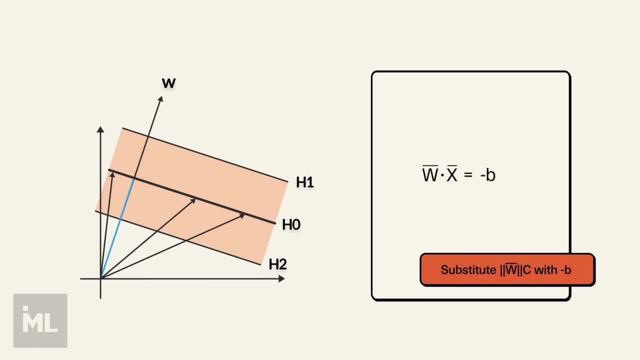 With negative b, we can get the function of the line H0, as w dotted x plus b is equal to zero, which is the equation for H0.. Here we only have two dimensions, so this can be expanded as the following function: In fact, this expression works for any number of dimensions. 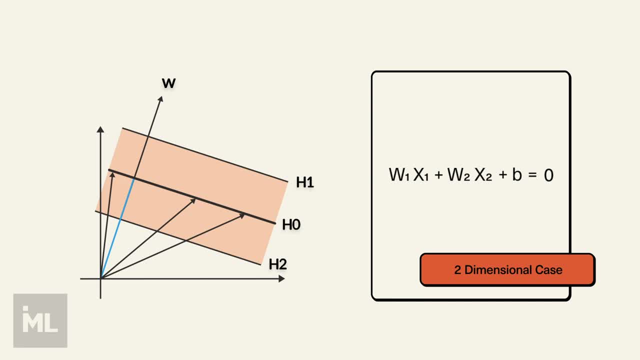 Once we have the expression of hyperplane, we can then use it to make predictions. For this example, if the expression for any unknown sample is equal or greater than zero, we predict it as a positive sample. Otherwise, we predict the unknown as negative. 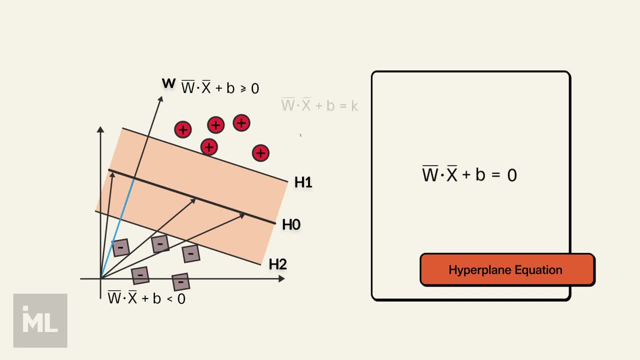 Similarly we can write the expression for gutter H1 and H2.. Here k is just another constant value and we can rescale w and b to make k is equal to 1. for mathematical convenience, As we have introduced before, SVM is a maximum margin classifier To find a way to express a margin or straight width here. 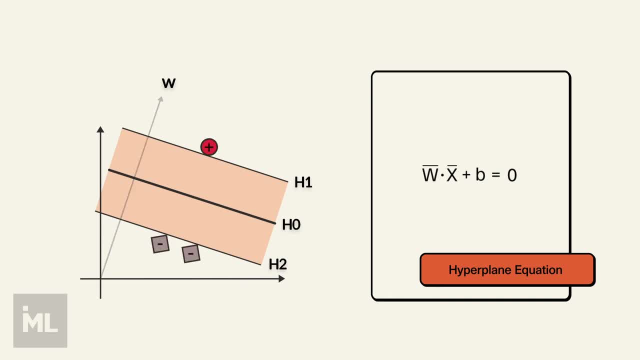 let's introduce two vectors, one x negative to a negative sample on the gutter H2, another one x positive to a positive sample on the gutter H1.. Now let's take the difference of these two vectors and dot product is, with the unit vector perpendicular to H0, we can get the expression of the width of the straight. 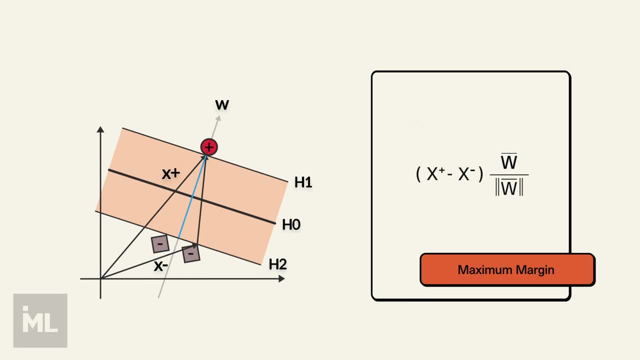 From previous derived function for gutter H1 and H2, we can get: w dotted x positive is equal to 1 minus b for the positive sample and w dotted x negative is equal to negative 1 minus b for negative sample. Let's substitute them back to the straight width equation and derive it. 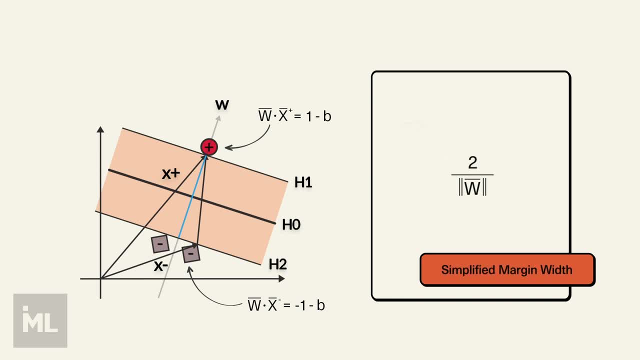 as 2 over the magnitude of w. In order to maximize this width, we thus need to minimize the magnitude of w. For mathematical convenience, it is equivalent to minimize 1 half times the magnitude of w squared, which also equivalent to 1 half times w dotted w. However, we cannot make the 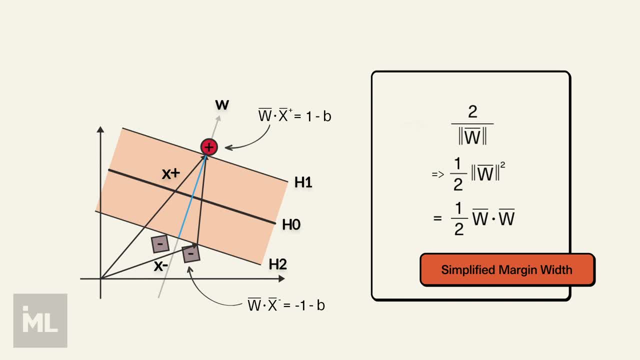 straight width arbitrary large. We can only expand the straight width under the condition that there are no data points between H1 and H2.. Mathematically this means for all the positive samples they should obey the constraint w dotted x plus b is greater or equal to 1, and for all the negative samples. 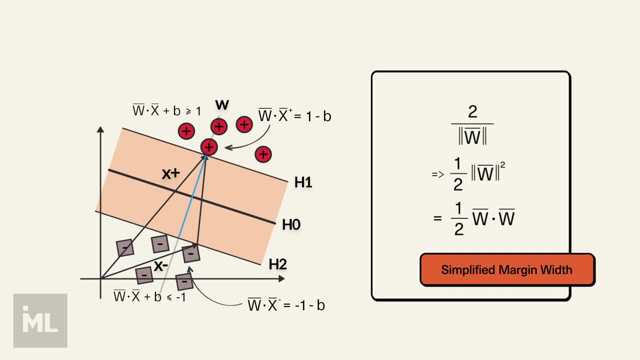 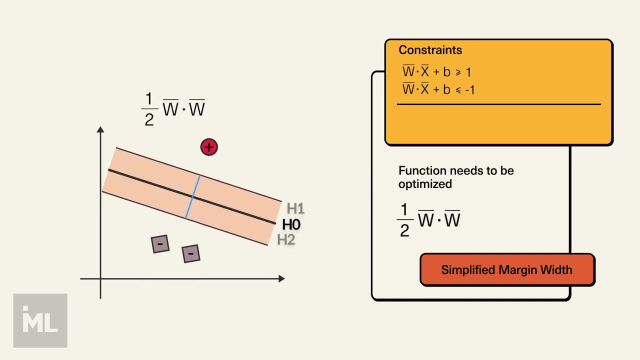 the constraint is: w dotted x plus b is less or equal than negative 1.. Now let's introduce another variable, y, to transform these two equations to make it more convenient from mathematical perspective. Here we assume y to be 1 for all positive samples and negative 1 for all negative samples. 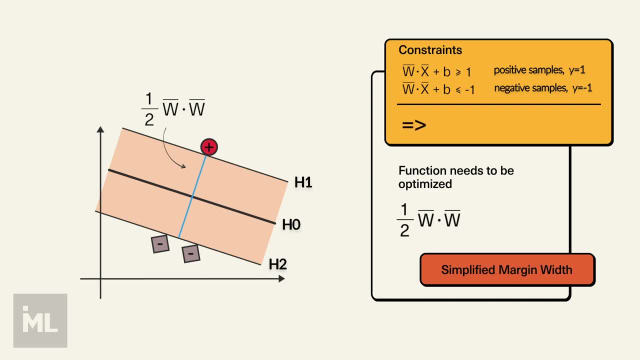 So the previous two equations can be rewritten as a single equation for all the samples. Let's revisit the problems we are trying to solve Here. we want to optimize the straight width 1 half times w dotted w, subjected to the constraint equation for all the samples. 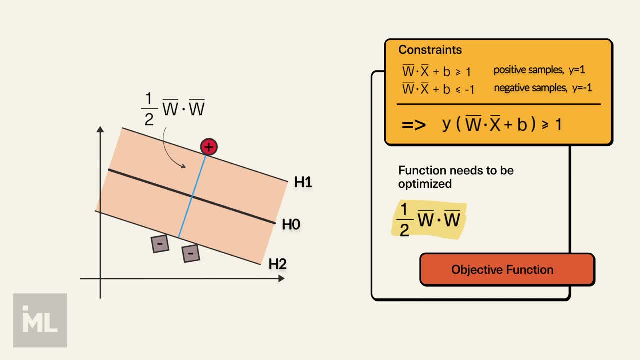 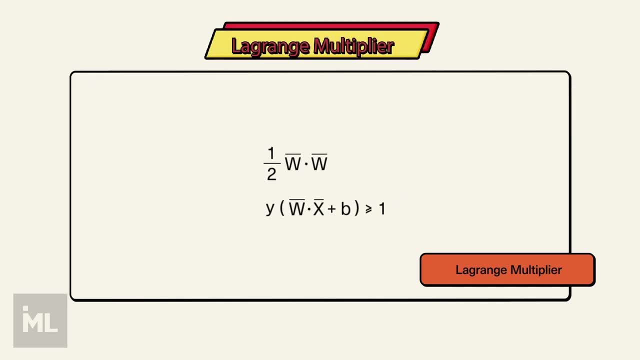 It is a constraint optimization problem and we have a powerful technique- Lagrangian multiplier- for this. If you are going to find the extreme of a function with a constraint, then we are going to have to use Lagrangian multipliers. This will give us some. 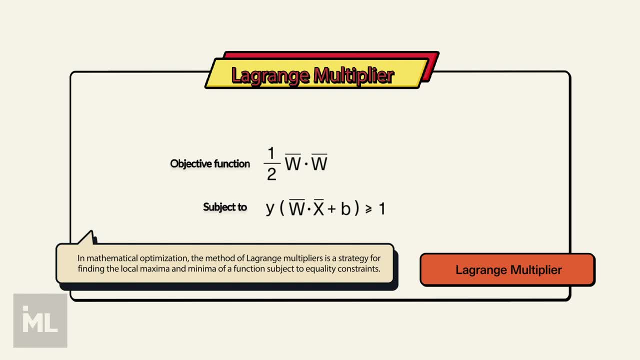 new expressions using which we can find the optimization of it without thinking about the constraints anymore. For this problem, the new expression can be written as 1 half times the w dotted w minus the summation of all the constraints, and each of the constraints is: 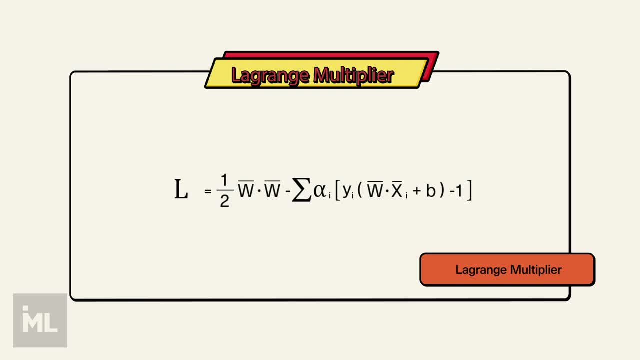 going to have a multiplier alpha sub i. What we are going to do next is to find the extreme of this new expression. Well, for this, we just need to find all the derivatives of this expression and set them to zero. The first equation is a partial derivative of. 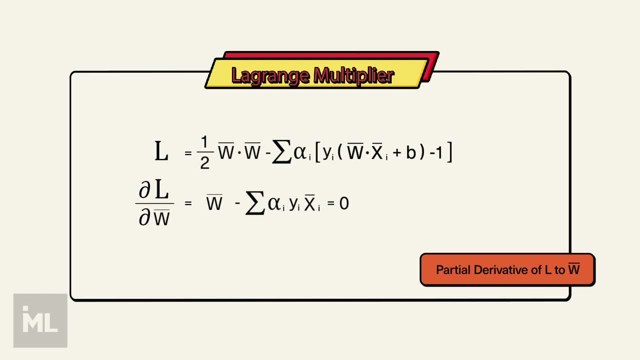 L the Lagrangian. with respect to the vector W, After setting it to zero, we can get the w equals to the summation of alpha sub i times y sub i times x sub i over i for all the samples. This is very interesting. It tells us the vector W can be obtained. 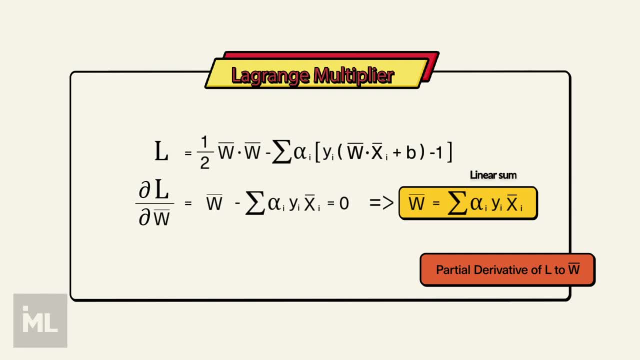 with a linear sum of the sample vectors. Actually, at the end of the optimization, a lot of alpha i is going to be zero and the nonzero alpha i correspond to the samples in the gutter, which is the support vectors. Now we should differentiate the Lagrangian with respect to b as well, which is going to 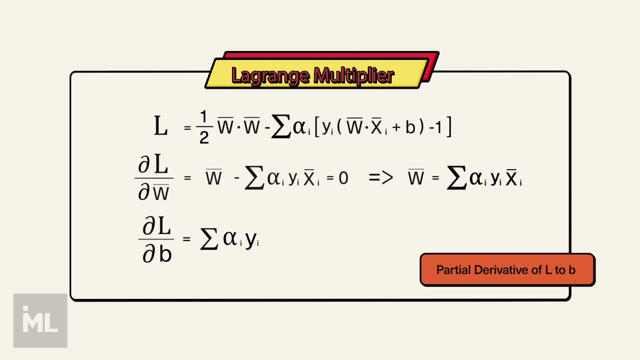 be equal to the sum of alpha sub i times y sub i. Also, at the extremum condition it should be equal to zero. Now we are going to plug the derived expression W back in the Lagrangian equation and the magic happens. here We can merge the. 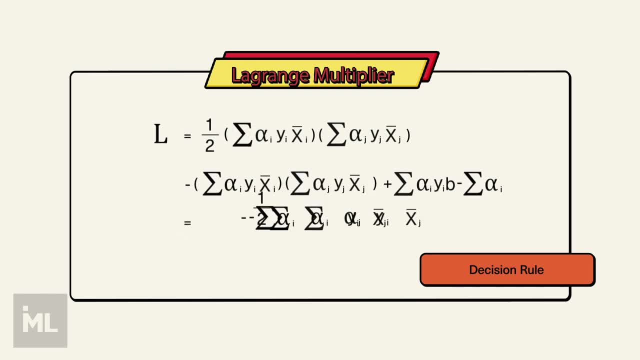 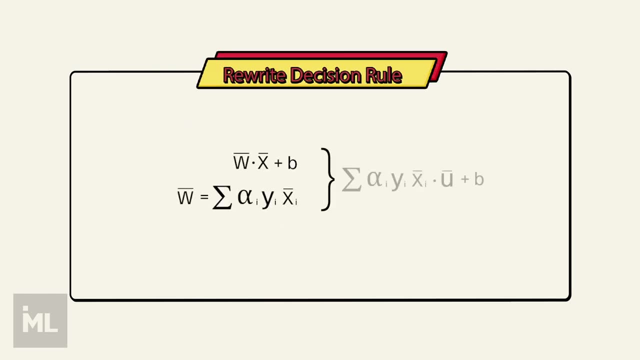 first term and the second term and rewrite the equation as a following one. What we've discovered is that the optimization depends only on the dot product of pairs of samples. So we can use the dot product of pairs of samples to substitute W. Now we can also substitute W. back to the decision rule, which is going: 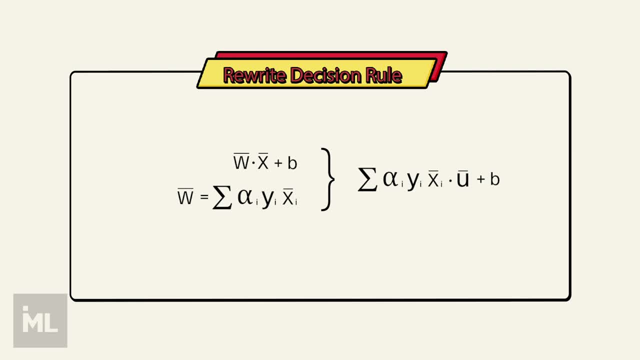 to be sum of alpha sub i times y, sub i times x sub i. dotted the unknown vector u plus b. If that is greater or equal to zero, then the prediction is a positive sample. Now we discovered that the decision rule also depends only on the dot product of those samples. 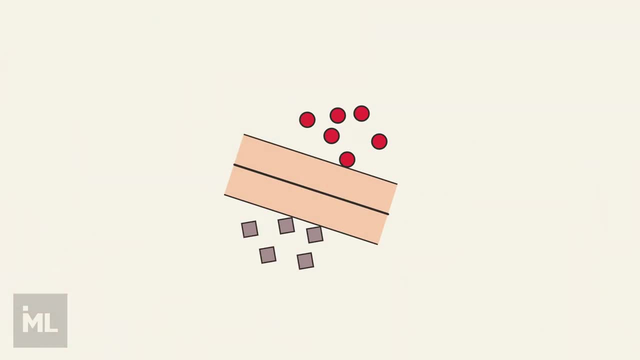 vectors with the unknown vector. Also, our previous discussion is based on the assumption that the samples are linearly separable and there is no outliers in the data, And the above SVM formulation is called hard margin SVM. What if there are some noise and outliers in the dataset? 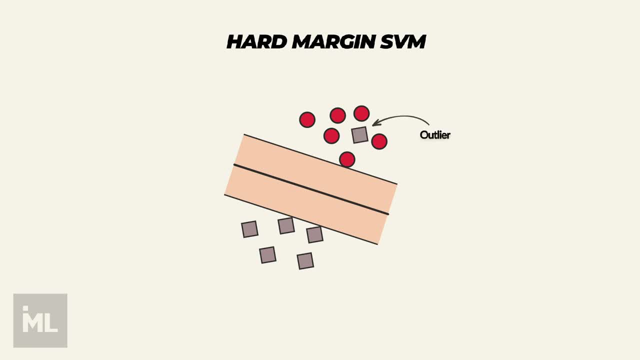 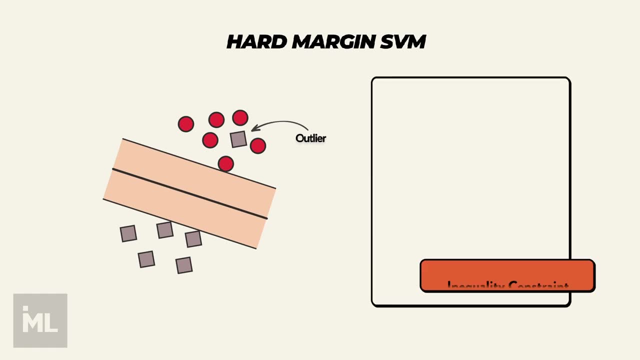 Then the hard margin. SVM simply cannot tolerate them and failed to find the optimization. Let's revisit our inequality example. Let's revisit our inequality example: constraint: here For the optimization problem to be solved, all the constraints have to be satisfied. In this part, we will talk about how to deal with this. 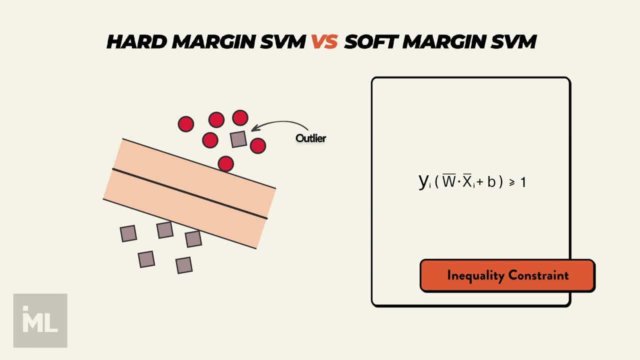 limitation using soft margin SVM. Basically, the trick is very simple. Let's add a slack variable, zeta, to the constraint of the optimization problem. It now becomes this equation with zeta: By adding these slack variables, when minimizing the objective function, it is now possible to satisfy the constraint. 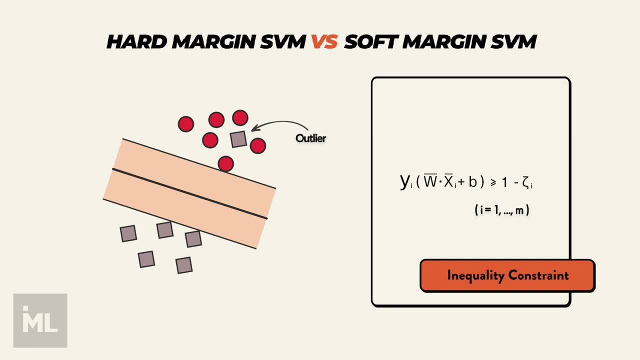 even if some outliers do not meet the original constraint. The problem is, we can always choose a large enough value of zeta so that all examples will satisfy the constraints. One technique to handle this problem is to use regularization, For example. if we want to solve this problem, we need to use 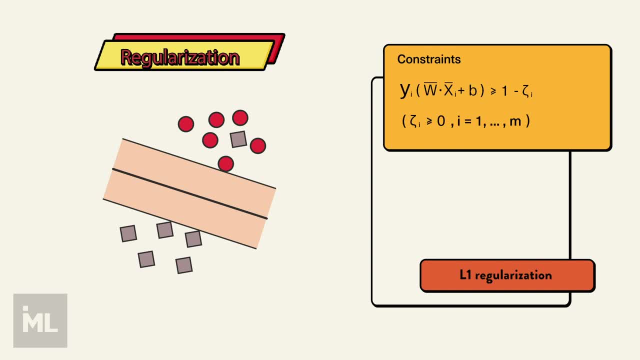 L1 regularization to penalize the large value of zeta. Now the regularization optimization problem becomes the following expression: Notice that the zeta here is always a positive number and the regularization parameter c determines how important zeta should be, which means how much we want to avoid. 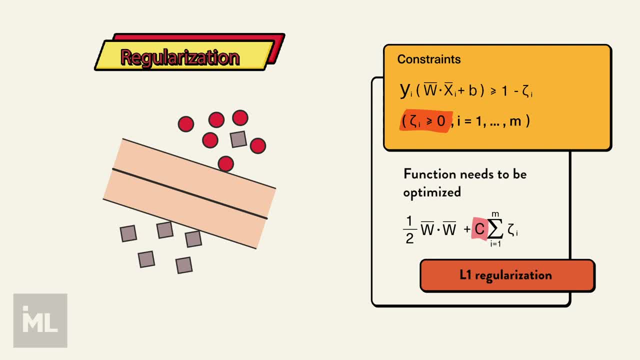 misclassifying each training example. A smaller c emphasizes the- the importance of theta, and a larger c diminishes the importance of theta. If we set c to positive infinite, we will get the same optimization result as the hard margin, SVM. So small values of c will result in a wider margin at the cost of some misclassifications. 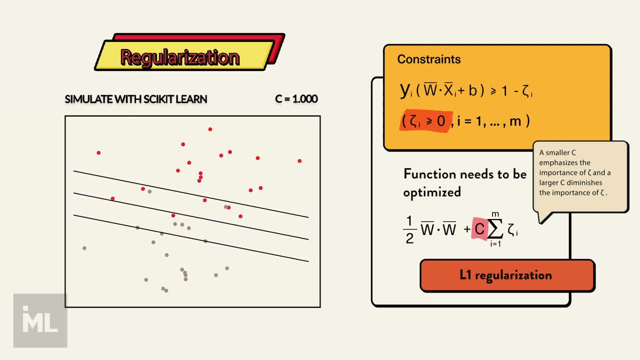 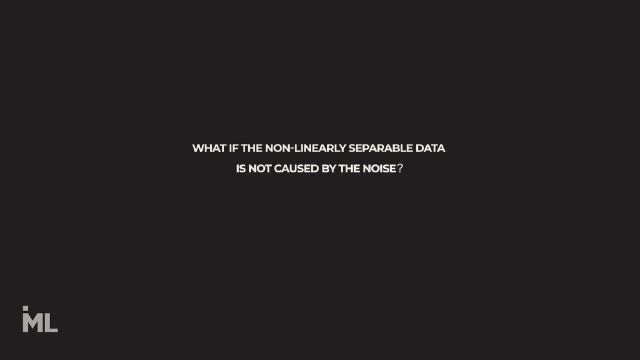 large values of c will result in the smaller margin and less tolerant to outliers. Now the soft margin. SVM can handle the non-linearly separable data with some outliers and noise. What if the non-linearly separable data is not caused by the noise? 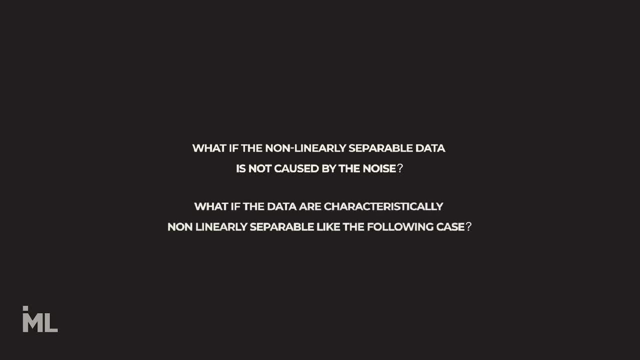 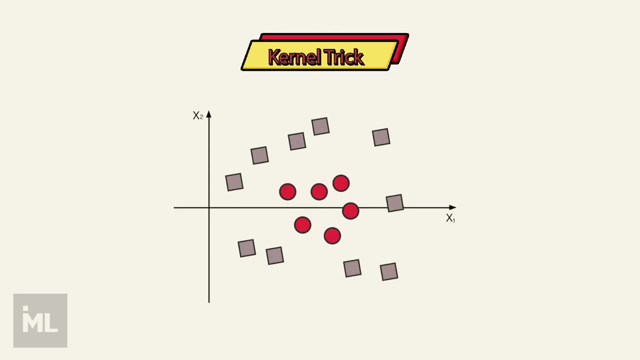 What if the data are characteristically non-linearly separable, like the following case? In this part we will talk about a technique called kernel trick to deal with this kind of problem. For this example, it looks like there is no easy way to. 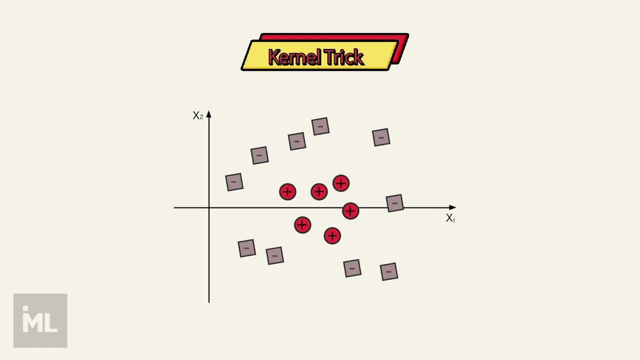 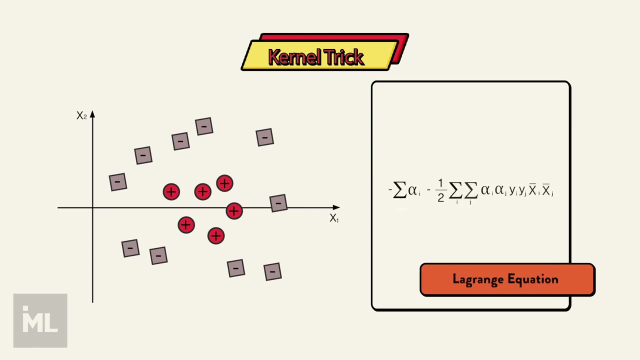 draw a line to separate the positive samples from the negative samples. However, if we transform the data from one space to another space, we would be able to find a hyperplane to separate the data. Now let's revisit our Lagrangian expression. 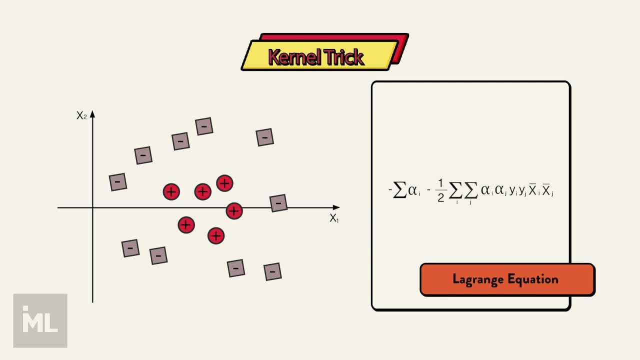 We find that the optimization only depend on the dot product of the sample- x sub i and sub j. So we could use any transformation function that can be expressed at the dot product of x sub i and x sub j. We call this function kernel function. 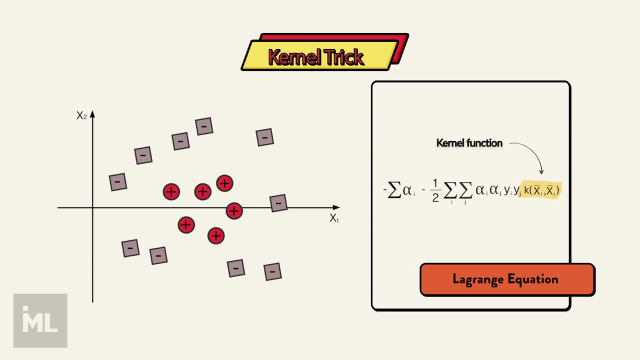 So the kernel trick is to define a kernel function k, and use it to replace the x sub i dotted x sub j in the Lagrangian expression. This is a small but powerful trick For these problems. we could write the kernel as: x1 sub i square plus x2 sub i square. If we plot these samples in the new space, a clear separation is possible. For this problem, we could write the kernel as: x1 sub i square plus x2 sub i square. If we plot these samples in the new space, a clear separation is possible.